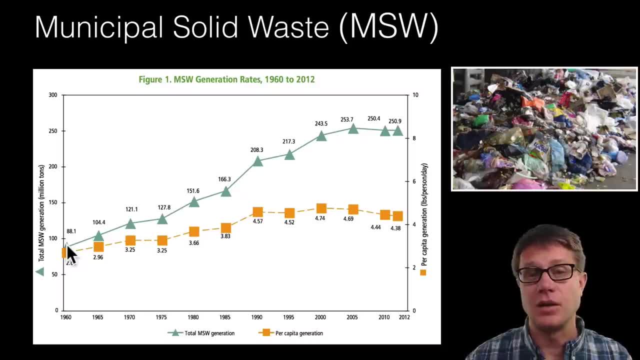 increasing from 88 million tons of MSW in 1960 to around 251 today. So you can see it is increasing over time and it is starting to level off as we start to recycle more of that. And this is per capita, per person, how much waste we are producing. So we are. 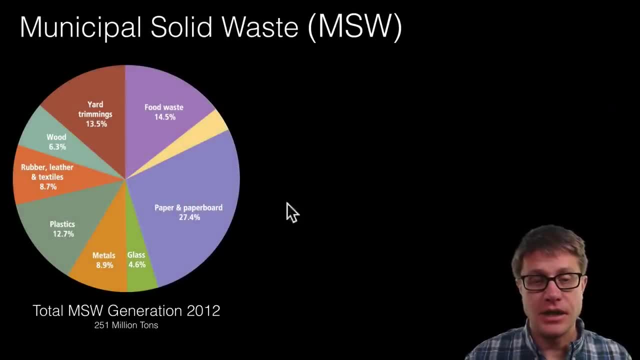 reducing. You should be familiar with what most of that waste is. This is from the EPA. It is generally going to be paper, food, yard trimmings, plastics, rubber, metals- 251 million tons per year. If we look at how much is actually disposed of, it is around 65% of that. This. 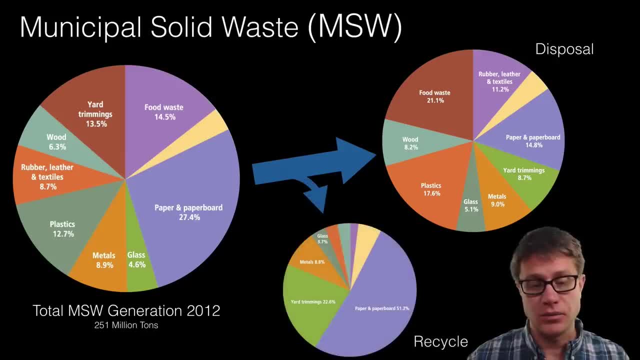 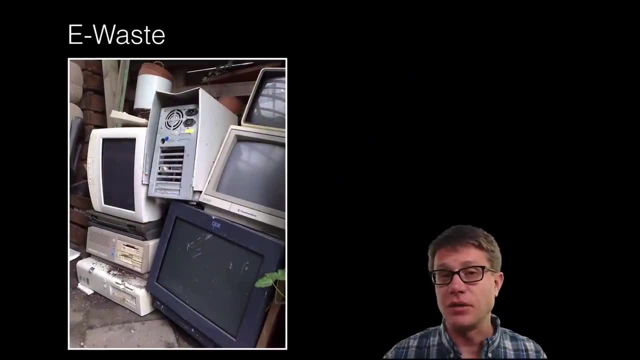 is to scale And the reason why is that we are recycling a lot of it. We are recycling especially the paper, the yard trimmings and the metal, Composting a lot of those yard trimmings- E-waste is a type of this waste. It is going to be the electronics We put. 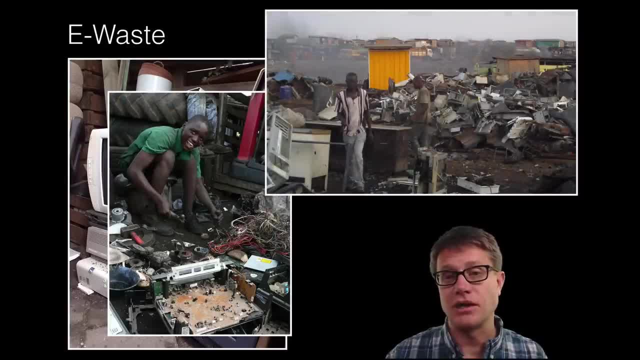 some of this in landfills. We put some of this in landfills. We put some of this in landfills. Unfortunately, a lot of it moves to developing countries where they recycle the parts of it And there are not standards, health standards- in place. So it is really 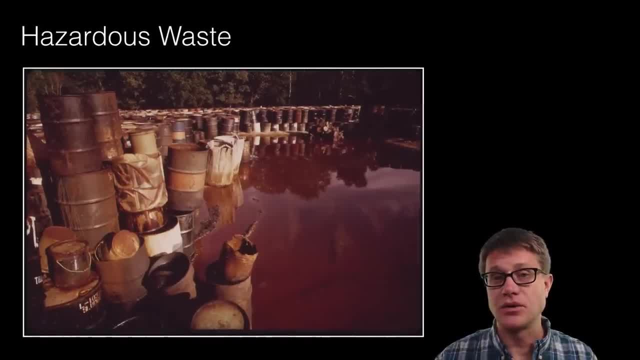 dangerous. And then we have hazardous waste. So chemicals that have been produced- Oven cleaner, for example, in your house- would be an example of a hazardous waste- And so we do not just bury that, because it gets into the ground supply. And so we have got regulations. 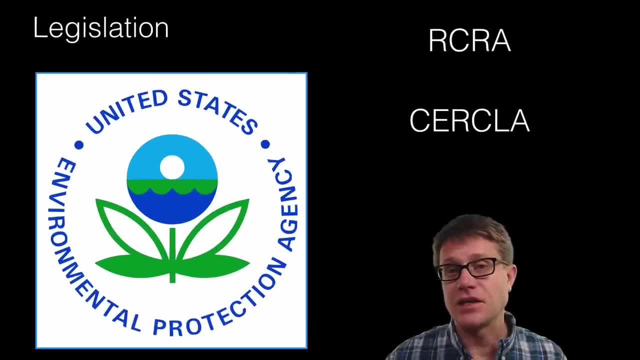 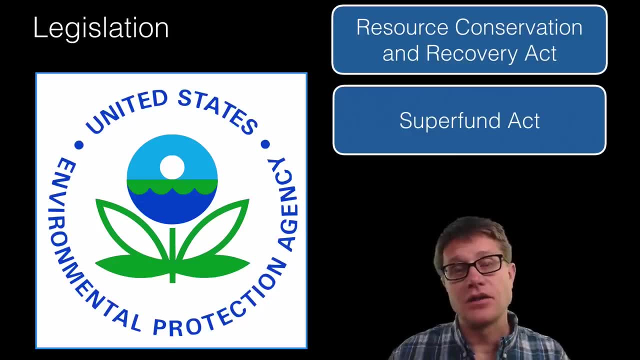 that make sure that we are storing it properly And that legislation could be broken down into RCRA and CERC law. RCRA is going to be the Resource Conservation and Recovery Act And then the Superfund Act. If we look at RCRA, that is going to regulate hazardous materials. 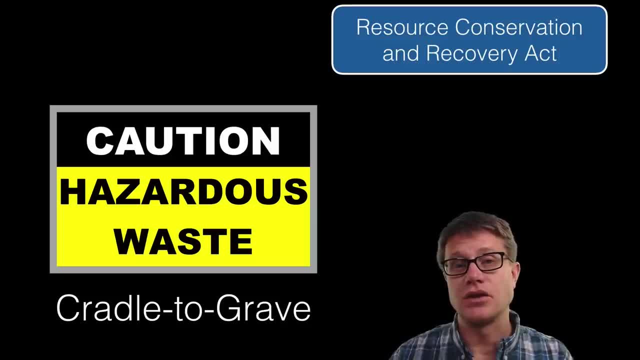 from cradle to grave, From the point it is created to when it is eventually stored. The way that works is we leverage taxes on the industries that produce these hazardous wastes and we can use that to help store them, And so, for example, that oven cleaner in your house. 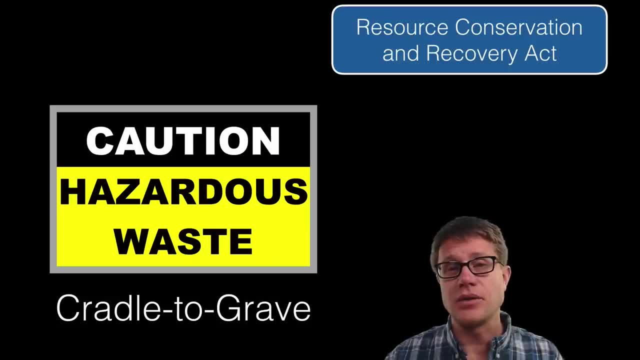 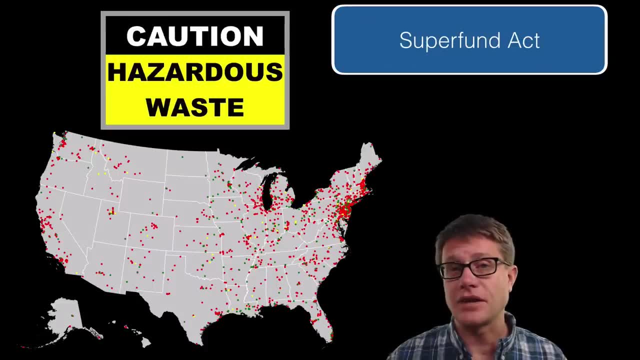 that you bought for five bucks is hazardous waste And so when you are done with it, if you do not use it- it is going to go to a place in your city where they can control that as a hazardous waste. The Superfund Act started with a very famous contamination. It is called Love Canal. This 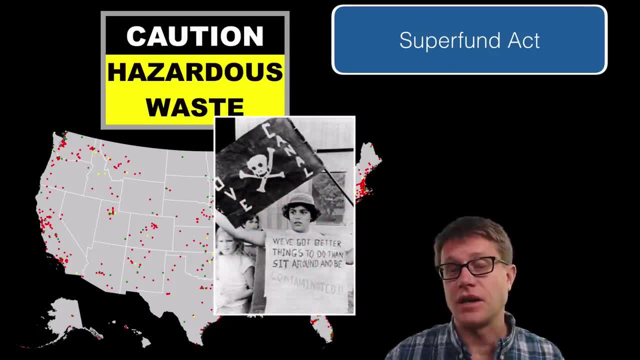 is in Niagara Falls, New York, And so back in the 40s and 50s a chemical company had been dumping hazardous waste and simply covering it, And that eventually that land was sold off to a school. Houses were built on top of it. We started to get birth defects, miscarriages. 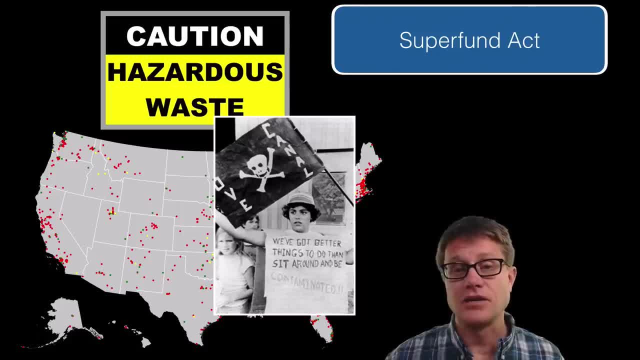 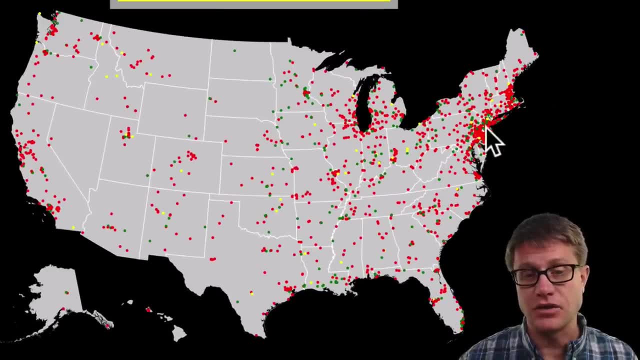 huge increases in illness, and they finally could trace it back to this. And so what the Superfund Act does is look at areas where we have huge contamination due to hazardous waste. All the red ones on here are Superfund sites. The green ones are ones that are done. 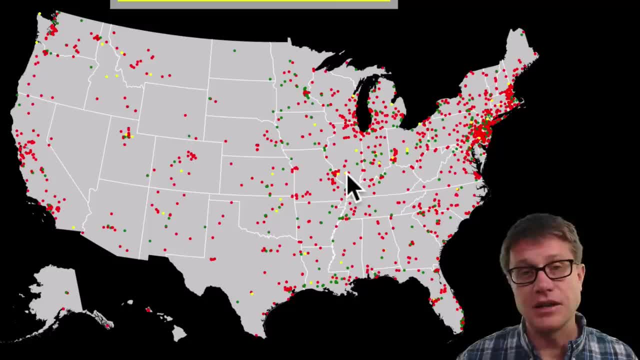 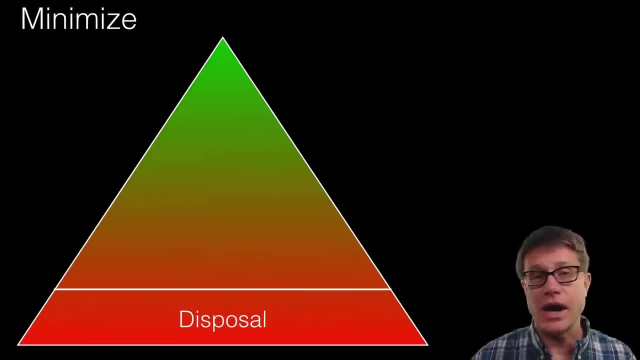 and the yellow ones are proposed Superfund sites, And so what we are doing is cleaning up the hazardous waste and holding those responsible if they are still around, those people who cause the contamination. And so how do we minimize the amount of waste We don't want? 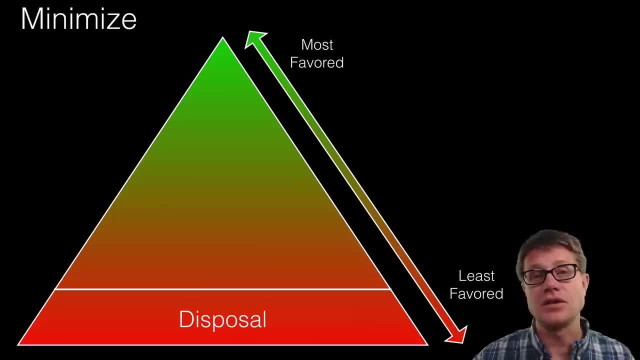 to dispose of it, And so we can think of it like this: From the least favored to the most favored, So we can dispose of it or we can get some of the energy from it, But we want to recycle it. if we can, We want to then reuse it, but we want to recycle the waste and we 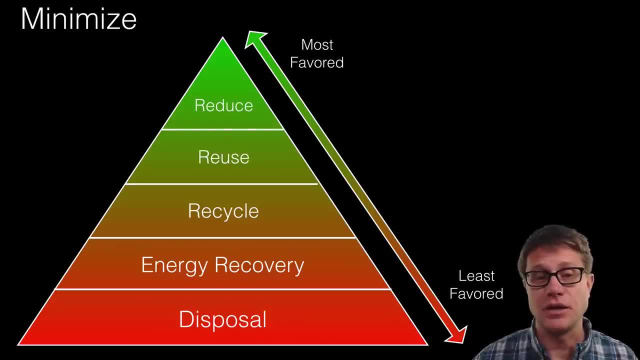 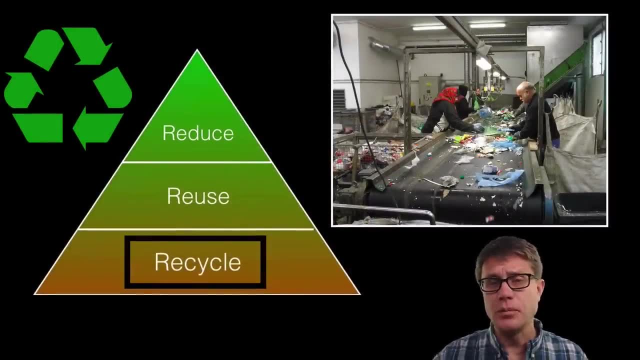 want to recycle the waste if we can. So what we are doing is we are cleaning up the hazardous, use it if we can and reduce it in the first place. So if we kind of break through those top three in recycling as this material goes to the landfill, we have people that can remove. 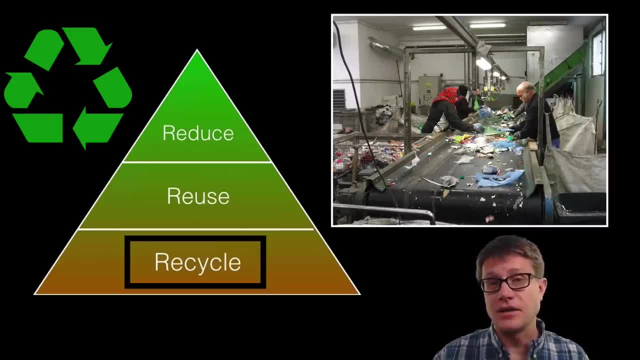 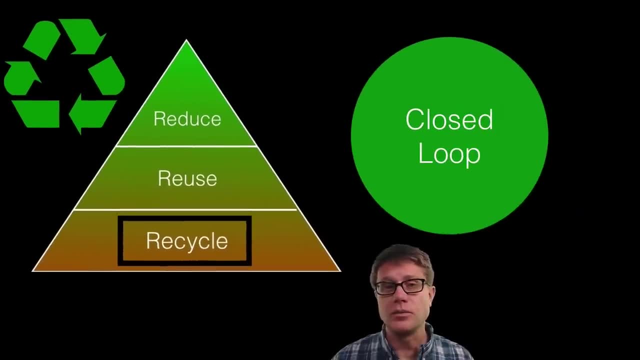 some of that recycling stuff that we can use again. Now that is pretty energy intensive, And so if we can have us do the sorting before it actually gets there, that is helpful. We have what is called closed loop recycling. That is where we take something like aluminum. 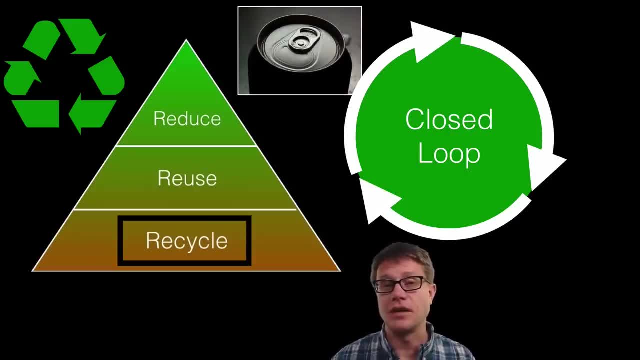 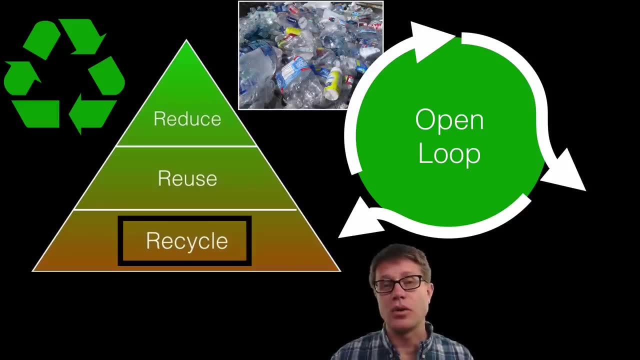 cans and we recycle that back to make more aluminum cans. And then we have open loop recycling And that is when we take something like plastic bottles and we can use that to make more plastic bottles, Or we can use it to make something like a polar fleece jacket. 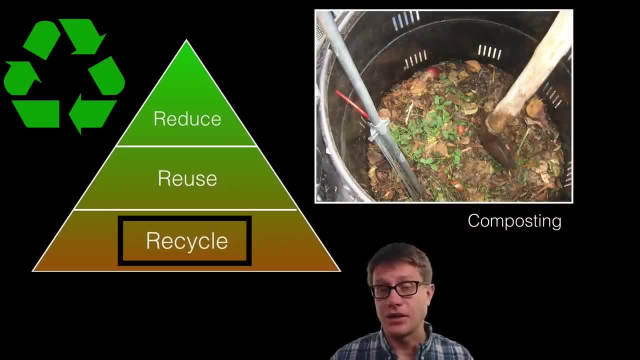 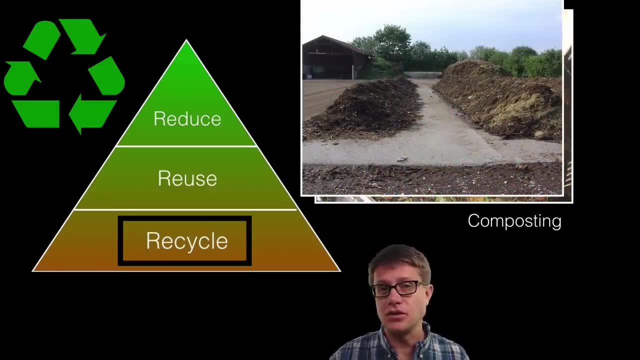 We also want to recycle nutrients. So composting in your backyard is a way to reduce the amount that goes to the landfill, And even at a large industrial scale. What we want to do is take those nutrients and put them back into the environment. 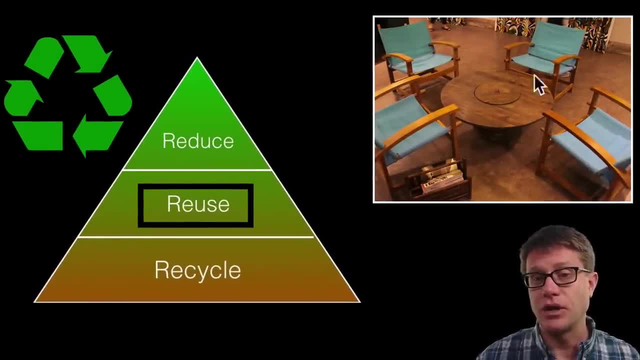 We can reuse that. So this is a giant coil that was. we had electrical coil that was wrapped around it And it is now used as a table. So if we can use things again, If you can give it to somebody else, Give it to Goodwill, You can sell it through eBay or Craigslist. Then we can reuse this. 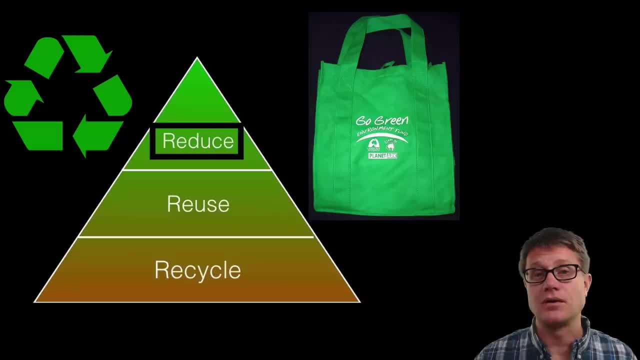 material, And at the best, we want to not even make it to begin with, And so if you have a bag that you take to the supermarket, then you do not have to choose. do I want plastic or do I want paper? You are not using either of those, And we can do it on an industrial. 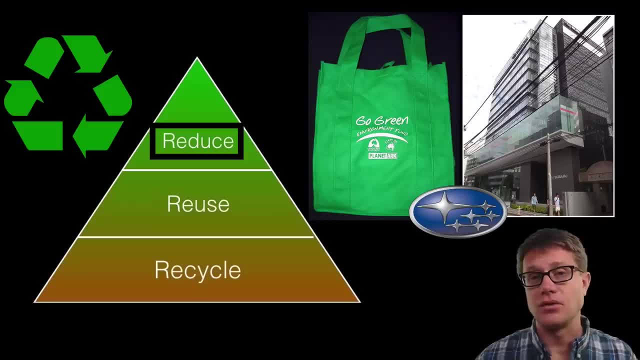 level as well. So Subaru, for example, is one of the first companies to go to a zero landfill policy. They are not putting anything in landfills. How do they do that? They are recycling, They are reusing materials And the little bit.